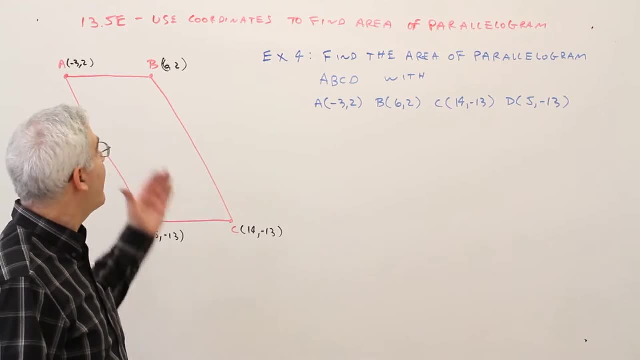 Welcome to video 13.5e. Use coordinates to find the area of a parallelogram. Here's example 4.. Find the area of parallelogram ABCD with the following coordinates: So I did a quick sketch. Again, you don't have to be super accurate, It's just for relative position. 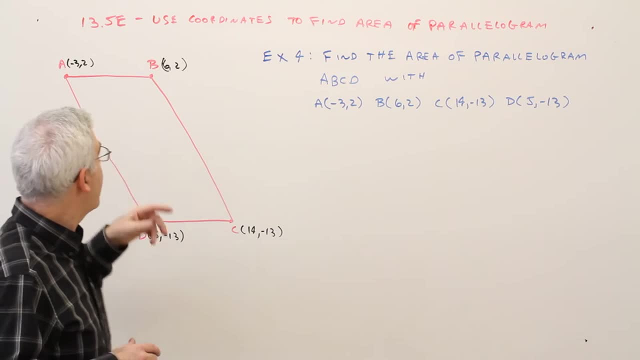 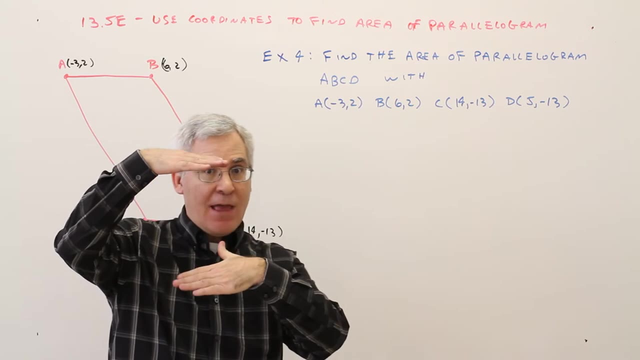 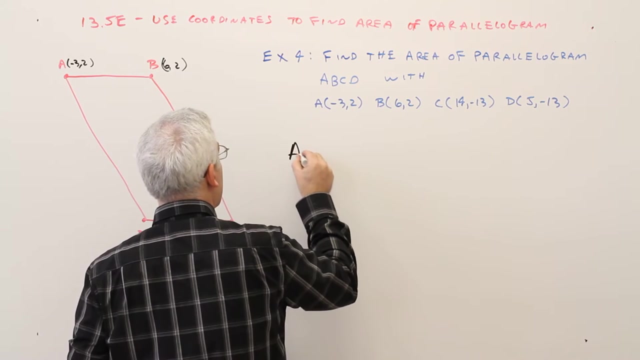 So ABCD. One thing to notice is that these two coordinates have the same y value, And these two coordinates have the same y value, So that means that they will be horizontal. Okay, So the area of a parallelogram is simply just the base times the height. 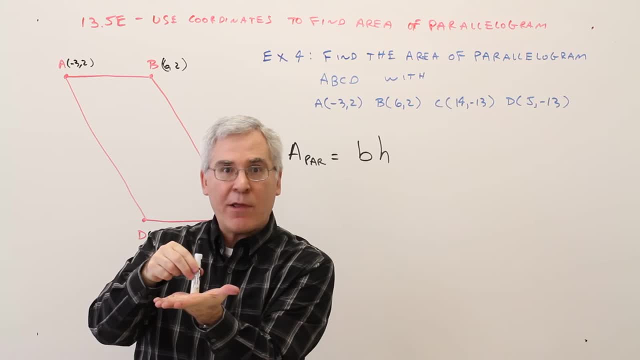 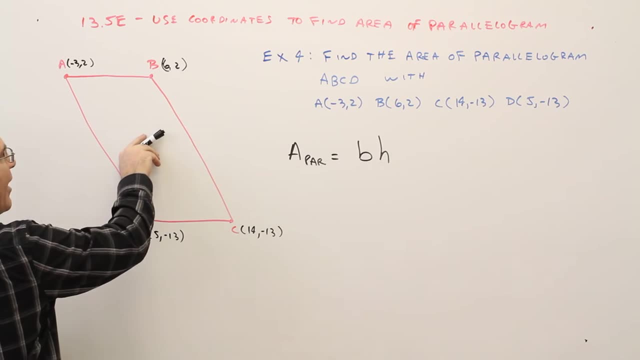 And once again, the base and the height must always be perpendicular, All right, So if you wanted to, you could call this the base, Then you'd have to find the height which runs on an angle. That wouldn't be so smart. 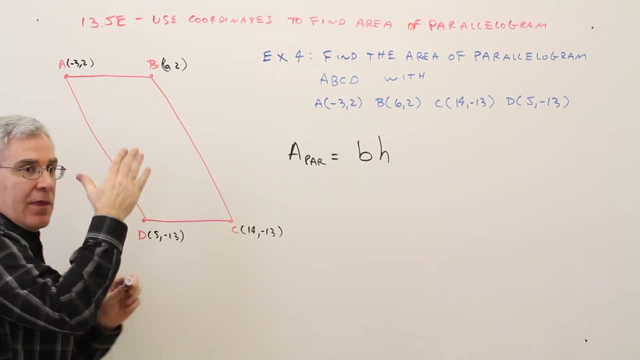 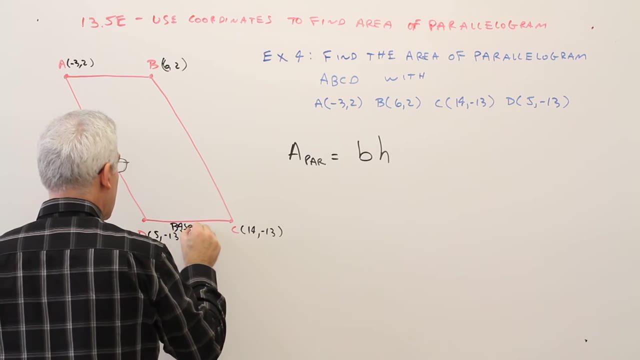 What we'll do is we'll call this the base, And the height is just simply the vertical distance which is easy to find, So I'll call this the base. You could use a distance formula. That would be not the best method. 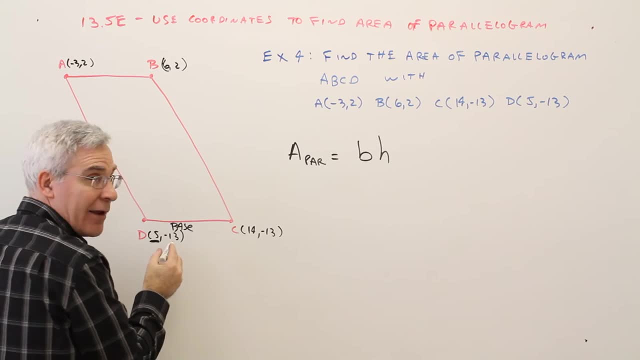 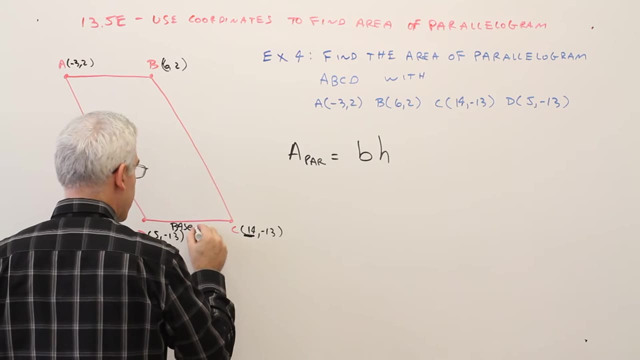 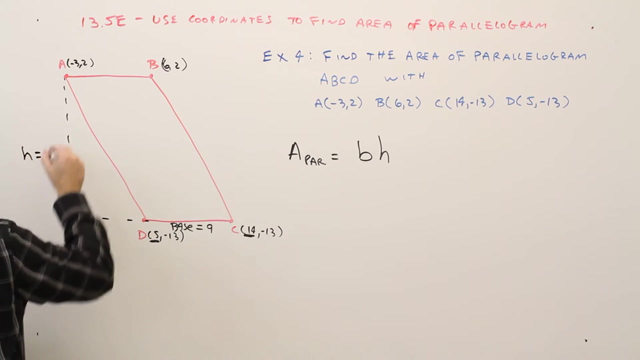 If you're just horizontal, you're just going from an x coordinate of 5 to an x coordinate of 14.. So that's going to be 9 units And the height Is simply that vertical distance. Notice again, this is horizontal. 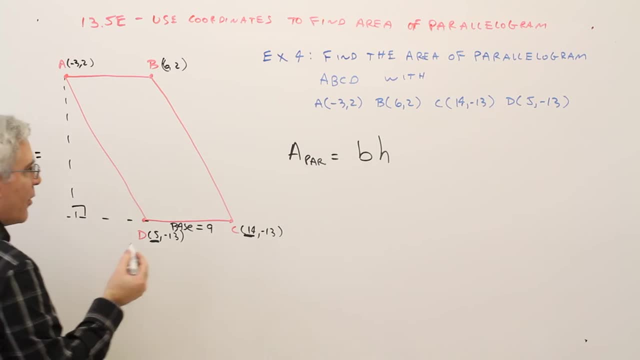 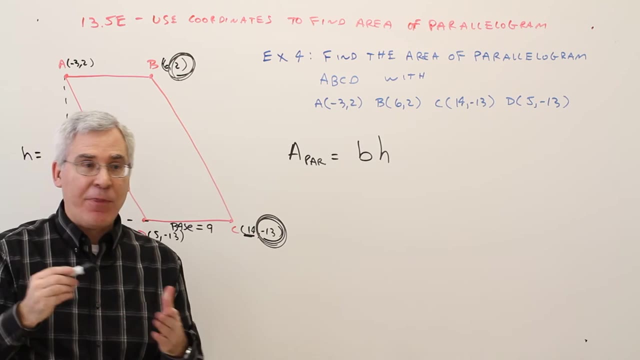 So something vertical would be perpendicular. So again, I could just go from this y coordinate to this y coordinate and find out that distance. So it's going to be 13 units to get to the axis And 2 beyond, that'll be 15.. 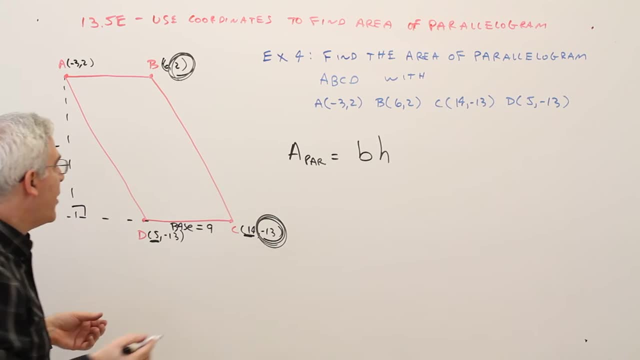 Okay, I've got the base, I've got the height, I'm good. So it's going to be the base, which is 9, times the height, which is 15.. What I could do is do some mental math. 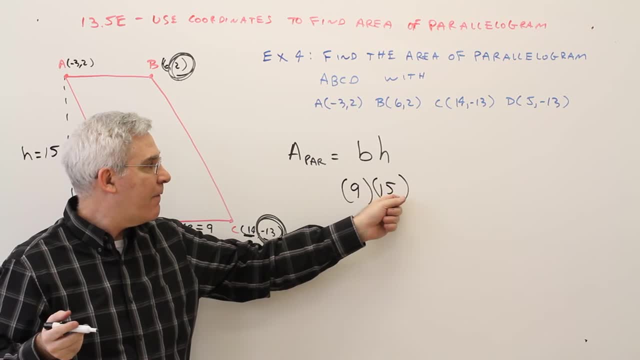 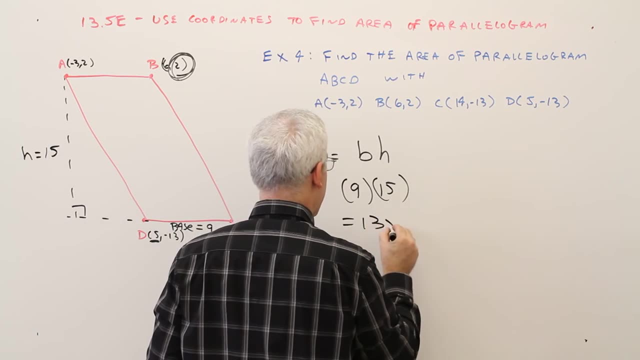 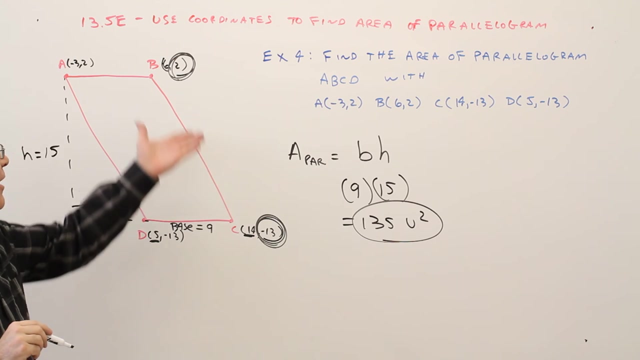 10 times 9 is 90.. 5 times 9 is 45.. 90 add 45 is 135.. And the answer would be 135 units squared. So there you have it: How to use coordinates to find the area of a parallelogram.